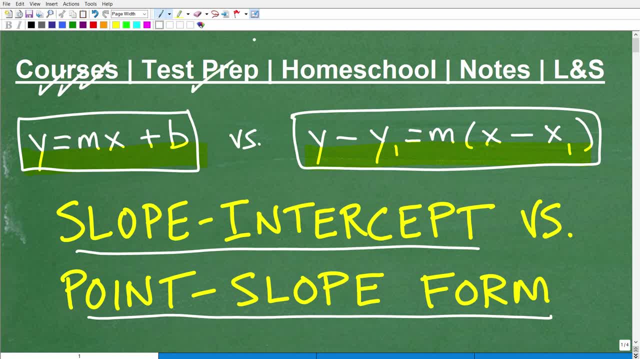 it will make a huge difference in your ability to understand mathematics. Also, if you're preparing for some sort of test, something that has a math section, like the ASVAB, SAT, ACT, GED, maybe a teacher certification exam, I have a ton of test prep courses that can help you out. If you homeschool. 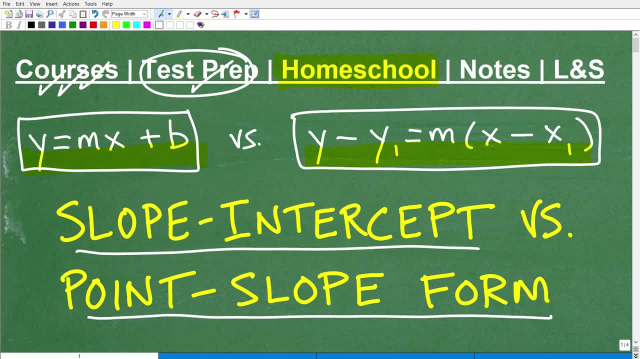 check out my award-winning homeschool programs for middle and high school mathematics. Very proud of this, I've been working with homeschoolers for years. Hopefully you have a pair of great math notes. Okay, if you're not taking great math notes, you need to start doing that immediately. 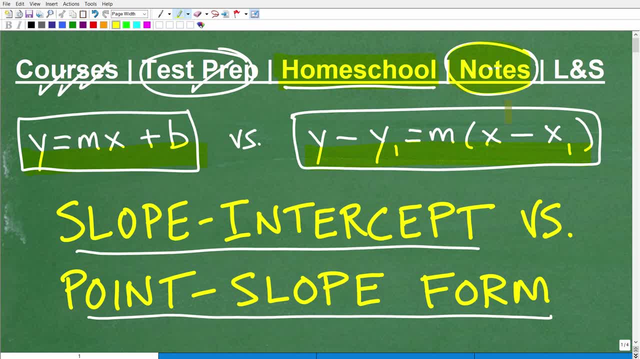 but you can use my notes. I'm going to leave links to those in the description of this video And if this video helps you out, don't forget to like and subscribe, as this helps me out big time. Okay, so let's get into the slope intercept form and the point slope form of a line. Of course, 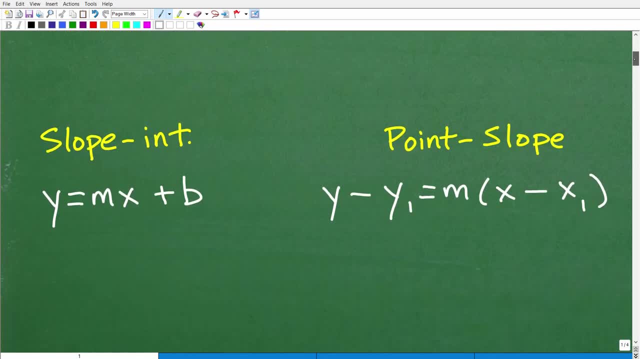 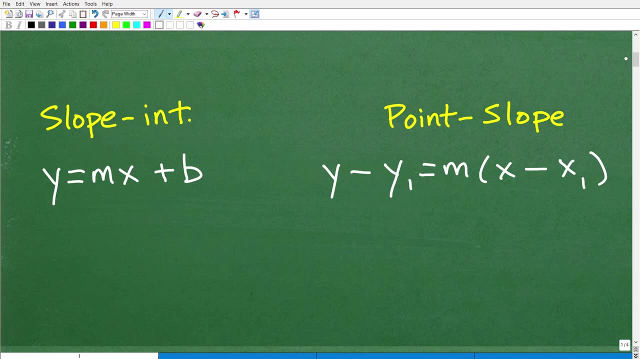 these are the two formulas, but let's go ahead and first kind of set this up. What is this? You know. what are we talking about here? What do these formulas have to do with? Well, this one right here, y equals mx plus b. the big topic really is something called. 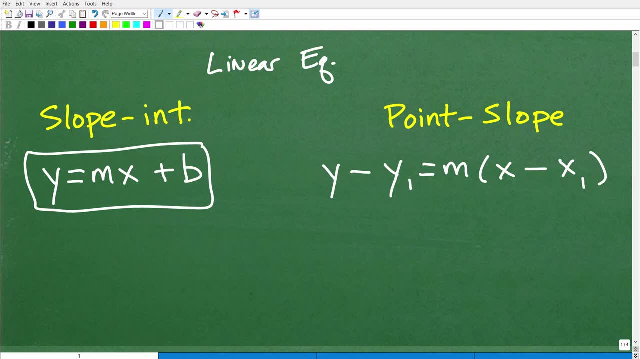 linear equations. Okay, this is a big topic in algebra and refers to kind of a lot of things, So linear equations could refer to. here's a linear equation: 2x minus 1 equals 5.. Solve this linear equation. This is a one variable linear equation But typically when you move beyond solving, 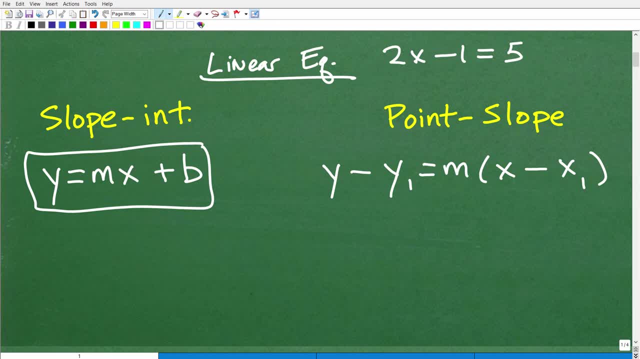 equations, and I'm kind of talking about pre-algebra algebra courses, algebra 1 courses you start getting into. hey, graph, the line y equals 2x plus 3.. Okay, you want to learn how to graph, But what are we? 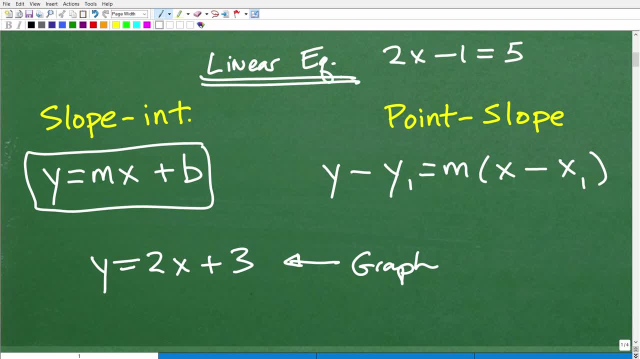 graphing. Well, we're still talking about linear equations, but we're graphing two variable linear equations. This word linear we've kind of- refers to line line equation. So this right here is the most common form to express an equation of a line. okay, ie something we can graph on the x. 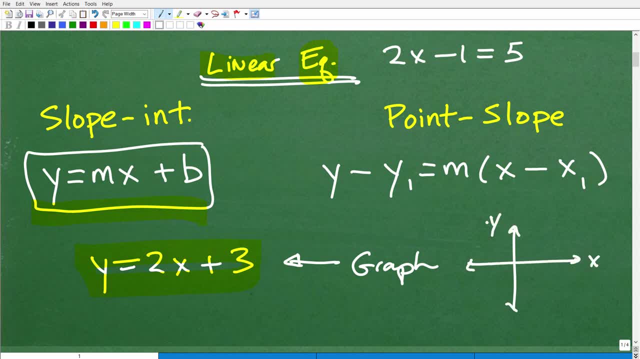 y plane. So here's x and here's y. I'm kind of being a little bit sloppy here, But if you wanted to graph a line, that would be a linear equation and that would be a two variable linear equation. And typically- okay, more often than not- it's going to be expressed in y equals mx plus b form. 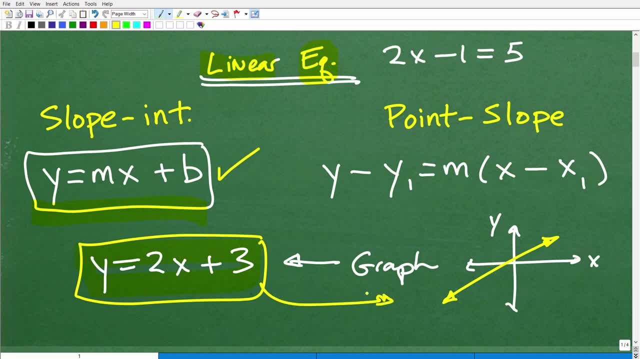 something like this we could graph on our nice little xy plane. So this is kind of the big picture that we're talking about. So you need to know how to graph a linear equation. So if you're thinking y equals mx plus b form, you need to know how to graph it. But the other part, 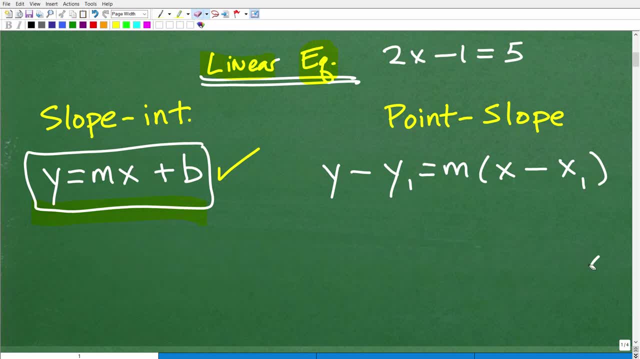 of studying linear equations is: hey, I'm going to give you a clue about a line. So, like hey, I know a line has a slope of one half and passes to the point three seven. can you tell me the equation of the line? let's find the equation of line. In other words, given this information, 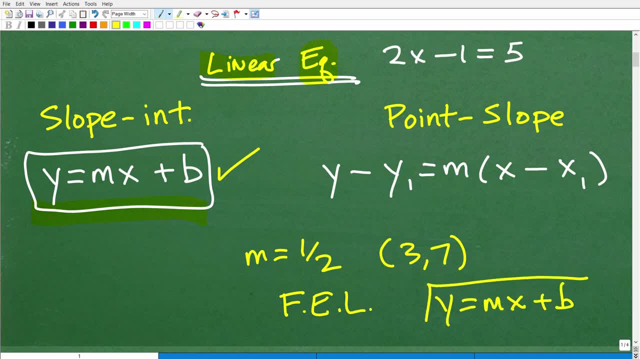 give me the y equals mx plus b linear equation that matches the line. So here's y equals mx plus b. this information Okay. so, given some hint hints about a particular line, find the equation to that line. So that's the kind of like the two primary things you need to understand when we're. 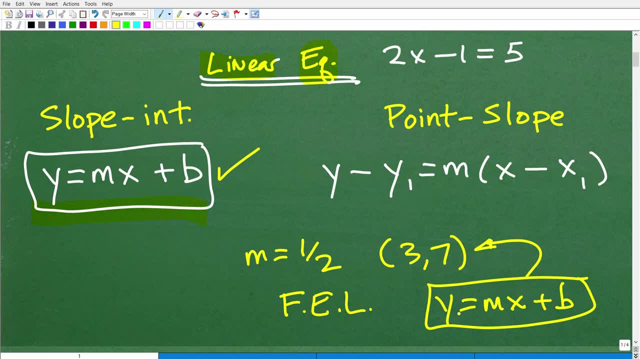 talking about the slope intercept form and a point slope form. Okay, and typically it's doing this flavor of problems finding the equation of line when you're going to be using this formula. Okay, so point slope formula is going to be super handy When we're answering this type of equation. 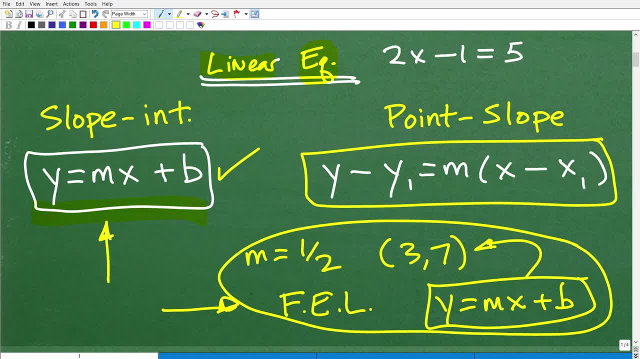 or this type of question. and then this right here, y equals mx plus b, is super handy When we are asked to kind of like graph a line or express a linear equation. we want to express this generally in y equals mx plus b form. Now there's other things here. I'm trying to teach you, like you know, two, three chapters. 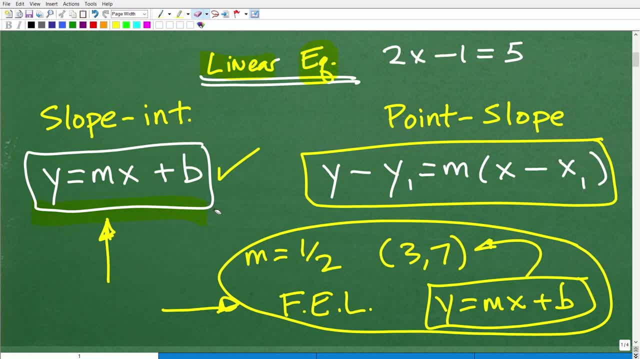 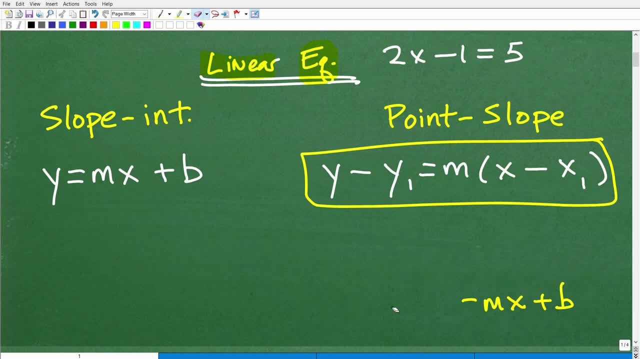 of an algebra course, You know, and it's impossible for me to do this, But I'm trying to give you the big points, because there's other things like standard form, etc. etc. But again, I just want to set this up because we are talking about the point slope. 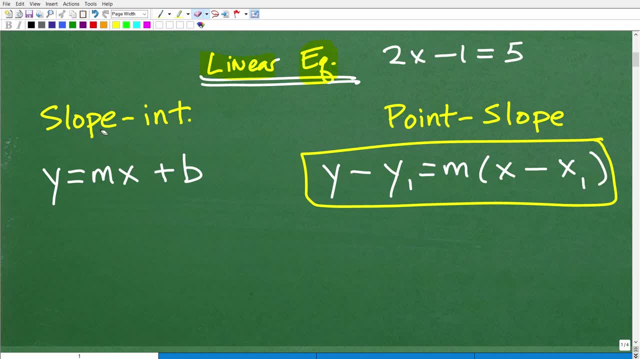 form or formula and the slope intercept formula or form of a line, okay, and it falls into the broader topic of linear equations. it's important that you understand the big picture because if you don't, this is how you know you're going to- not, you know- end up comprehending all this. 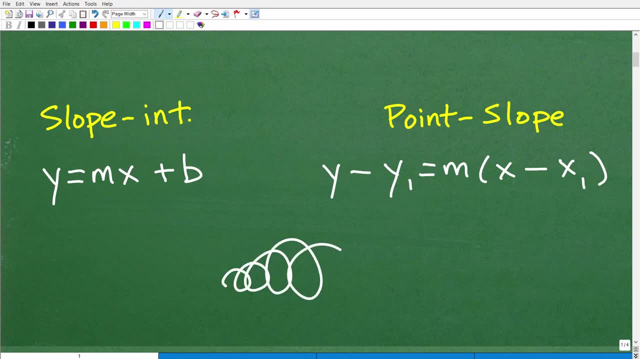 material, because you know, in algebra you're going to get thrown a lot, a lot of information, So we're not keeping up where all fits in. it will become confusing, Okay, so I wanted to set the stage there for the 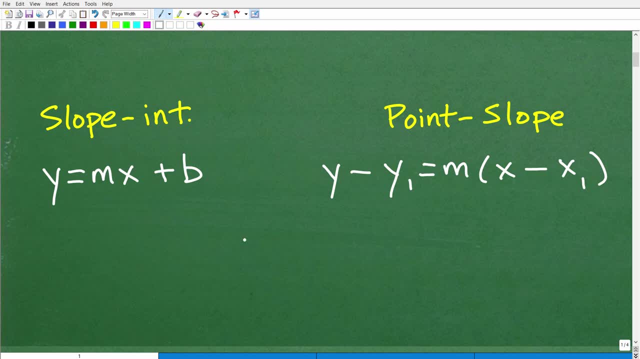 slope intercept form and a point slope form of a line. Now, another thing you need to know is this: if I'm trying to find the equation to a line, you need two pieces of information at a minimum. okay, you need the slope of the line, the M. okay, hopefully you have a good understanding. 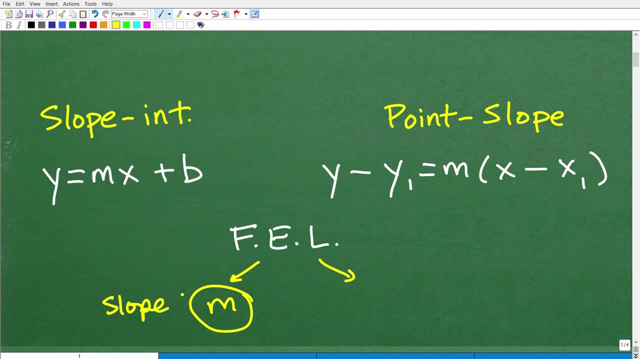 of what the slope is. If you do not, you definitely want to check out my additional videos on my YouTube channel on slope. I have a ton of them. or, better yet, just check out my math help program: my algebra course, pre-algebra, algebra, two course, any of those. I teach this big time. 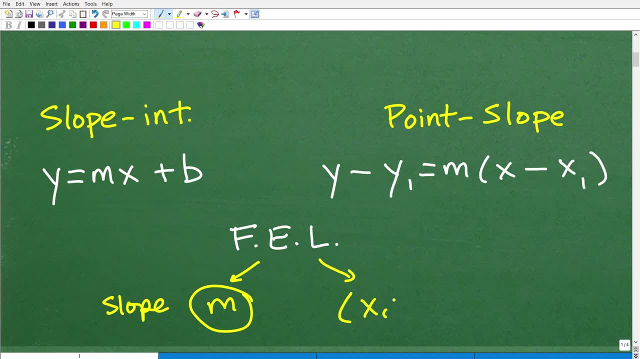 Okay. so you need to have the slope, okay, and you need to have at least one point that's on the line. okay, at least one xy point that's on the line. Now let's suppose you were asked to find the equation of a line and the question goes like this: find the equation of a line that? 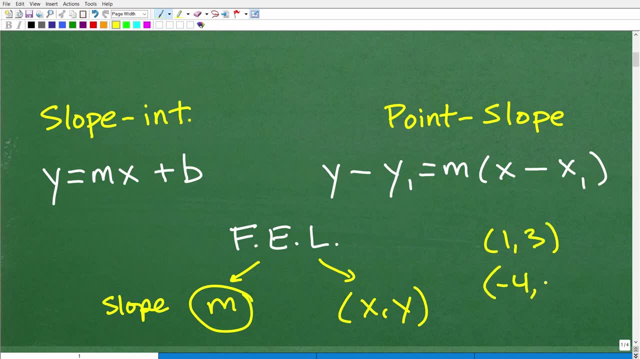 passes through the point 1, 3, and negative 4, 5.. You're like whoa. okay, I have two points, I don't have a slope, I just have two points. could I find the equation to this line? Yes, you can, because 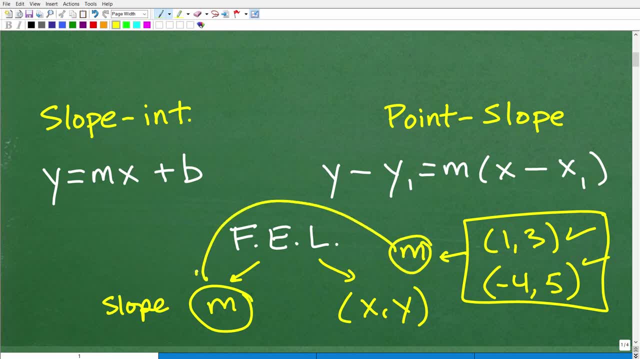 given these two points, you can find the slope. okay, so you can find the slope, but we need at least one point and you can. for this particular problem, you can use this point or this point, doesn't make a difference. okay, so I'm kind of quickly going over a lot here, because when we're 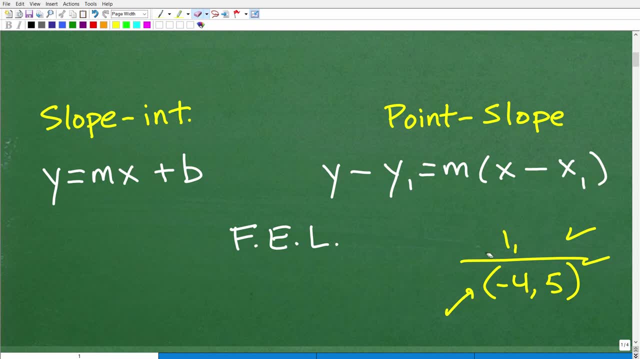 talking about the slope-intercept form and the point-slope form of a line. you need to understand the context of why we're learning this, okay, and that's what I'm kind of doing right now. Okay, so now let's get into the slope-intercept form. 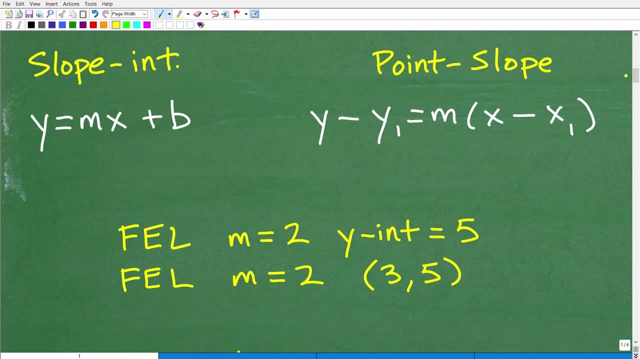 and point-slope form and I'm going to keep my focus primarily to finding the equation of a line. okay, so hopefully you understand how to graph a line. If you do not, again check out my videos on my YouTube channel or go to my algebra course, All right. so find the equation of a line, Let's. 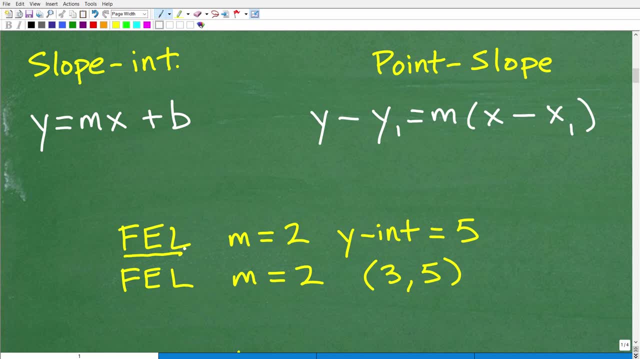 take a look at this first problem. So we want to find the equation of a line. Now, this here is the equation of a line. Typically, we're looking for the y equals mx plus b form of the line, the slope-intercept form of the line. okay, so to answer this question, we're going to take 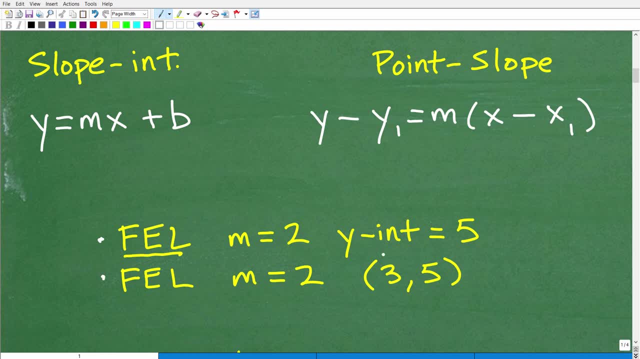 these are two separate questions. To answer these questions, you can use both formulas. okay, so to find the equation of a line, you can do all your problems using this formula. okay, the slope-intercept formula. and let's just go ahead and define something. Why do we call this? 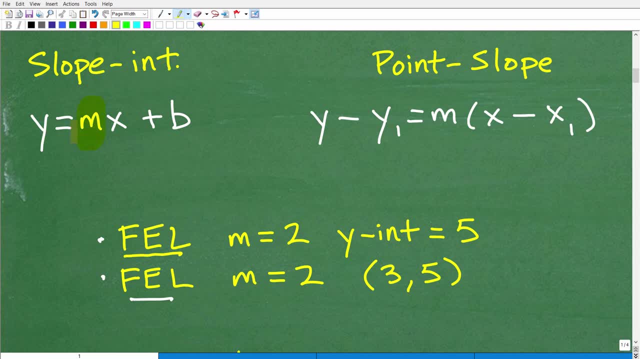 the slope-intercept formula. Well, the m is the slope, y equals m, m is the slope and the b here is the y-intercept. okay, this is the y-intercept. we just call it. that's a b, it's not a six. it looks kind of like a six. 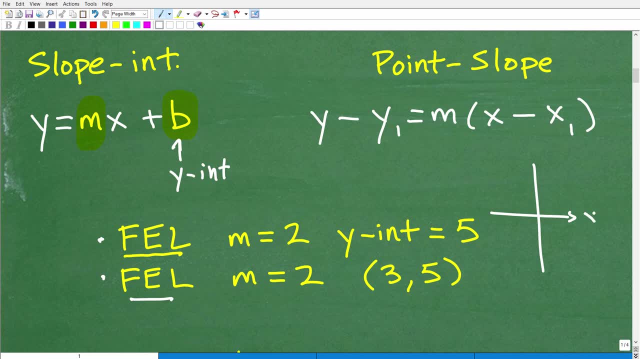 but that's the y-intercept of a line. So here, here's the x-axis and here is the y-axis. If we have a line that's chopping like going like this, this point, here that's crossing the y-axis, that's the y-intercept. 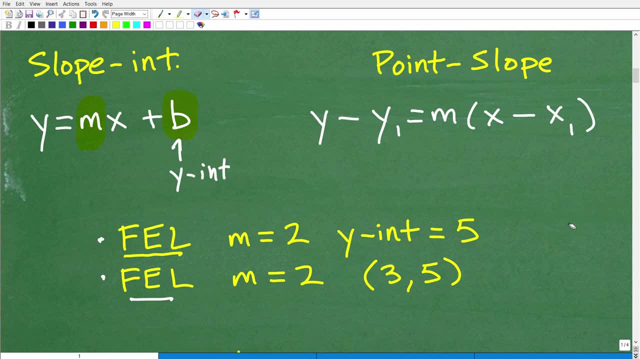 Okay, all right. so again, I really want to break this down thoroughly for you, so if any of you have been confused about this, you will not be confused by the time I'm done with this little video. All right, so this is a slope-intercept formula line again. 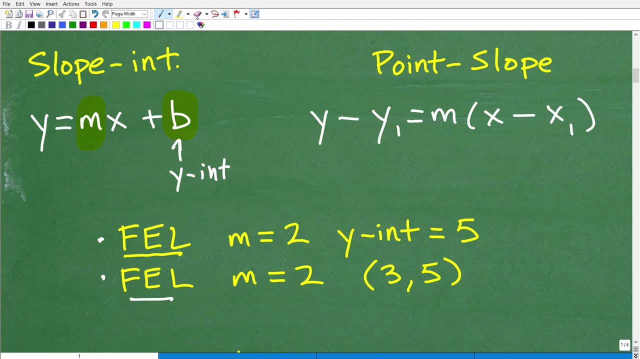 slope and y-intercept, or we just refer to it as the intercept. Now again, you can find the answer to the finding the equation to a line. you can use this formula all day long. okay, Now for some problems. you want to use this formula and I'm going to get to this in a second. 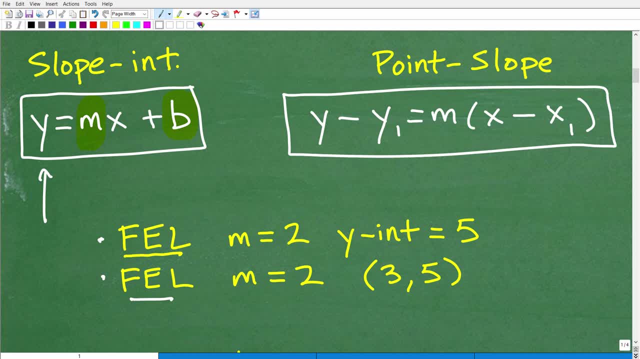 but I'm going to tell you right now the preferred formula to answer finding the equation of lines. I want you to think of using the point-slope formula. So I'm going to do a problem using the slope-intercept form. We're actually going to talk about these problems here in a 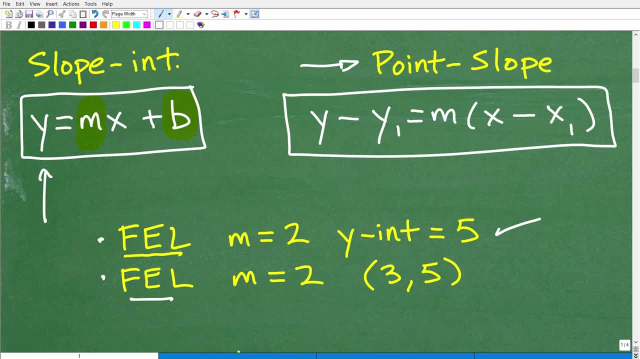 second, but I'm going to go over how we do, how we answer these questions using both formulas. Okay, but you have to be kind of smart about this. So let's take a look at this first question. Let's find the equation of a line with a slope. 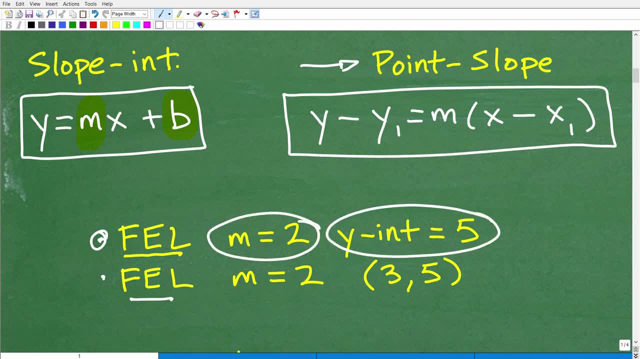 of two and a y-intercept of five. So, given these two formulas- okay, now I haven't even showed you how to use these formulas- Which formula would we choose? Okay? well, the obvious answer would be this one. okay, because to get the right answer for this formula, all I need is the slope and the. 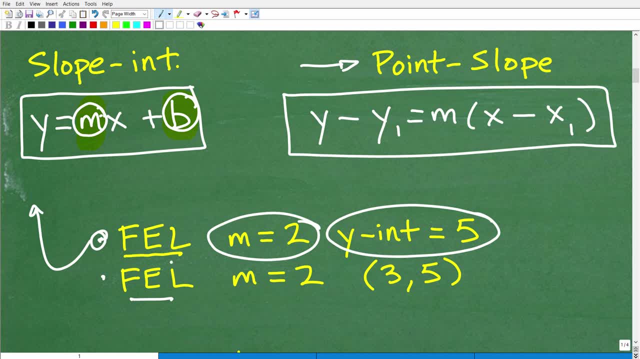 y-intercept. Here I have the slope and I have the y-intercept. So what's the equation of a line that has a slope of two and a y-intercept of five? Well, I'm going to take a look at this first question. 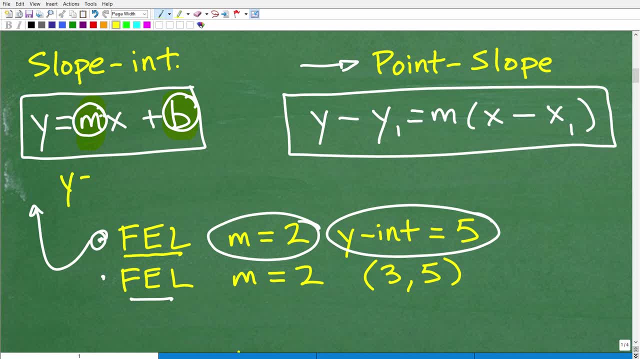 Well, you just go right over here. It's like as easy as this. Y equals well, the slope here is going to be two. Then I have x plus my y-intercept, that's my b is five. Okay, so right here is the. 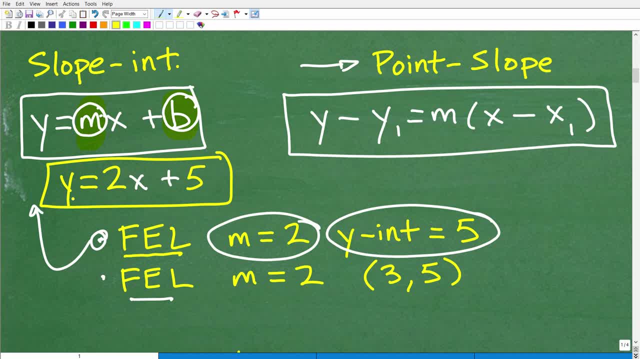 equation y equals two, x plus five. is the linear equation or the equation of a line that has a slope of two, okay, and a y-intercept of five. It's like one, two, three, Okay. now I could do, I could have answered this question by using this formula, but that wouldn't be smart, okay, So you. 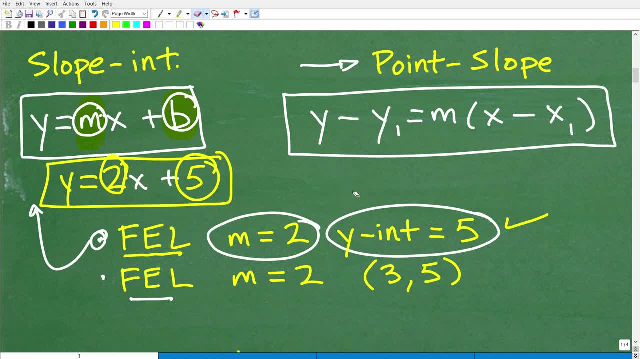 need to know both formulas, and that's what I'm kind of doing: I'm trying to compare and contrast these formulas for you, All right. so anytime you're asked to find the equation of a line where you're given the slope and the y-intercept, always use the slope-intercept form. It's just the most. 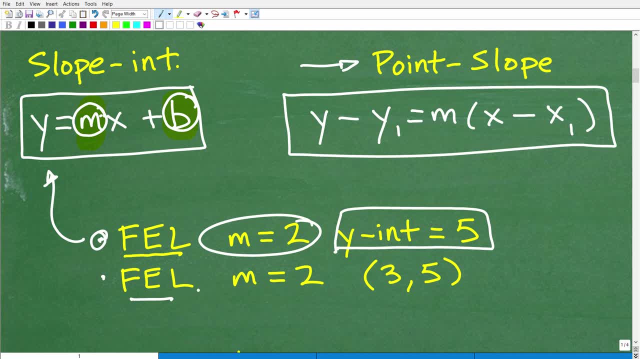 direct way to answer the question. Okay, now let's take a look at this problem. here We have slope of two and we have the 0.35.. Okay, in other words, we have a line, We want to find the. 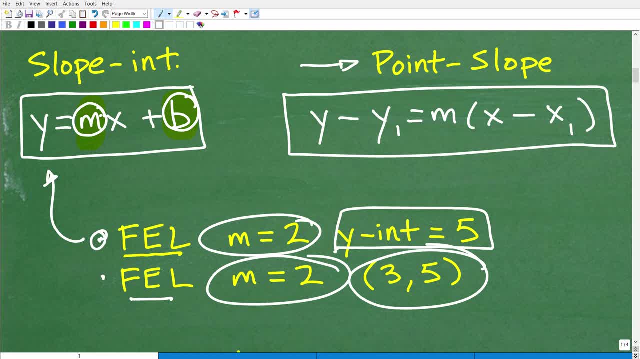 equation of a line that has a slope of two and passes through the 0.35.. To kind of visualize this, let me see if I can kind of graph this. Here's the x-axis, Here's the y-axis. So the 0.35. 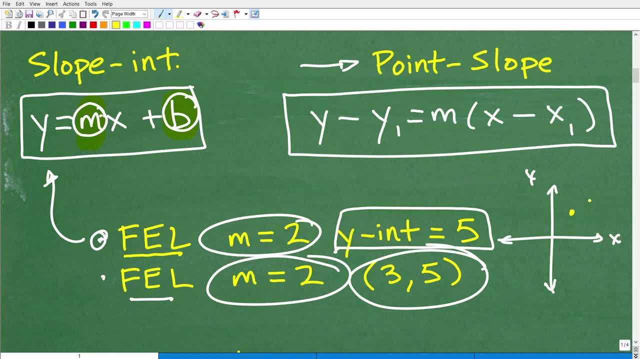 might be like right here. Let's say, this is three, five and our line has a slope of two, So it might something like this: okay, so here is our line, it has a slope of two, okay, and it passes the point three, five. we want to find the equation, the linear equation, and the linear equation will always be. 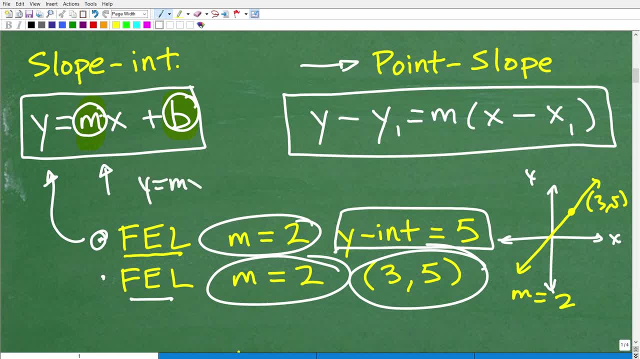 expressed in slope intercept form. y equals mx plus b form. okay, so our final answer. typically we want to express it in this form, but that doesn't mean we always use that. we're going to use this formula. we're just going to write our final answer in this form, okay, so so these type of questions, 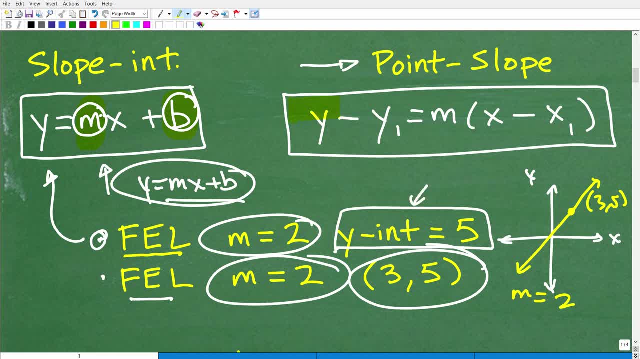 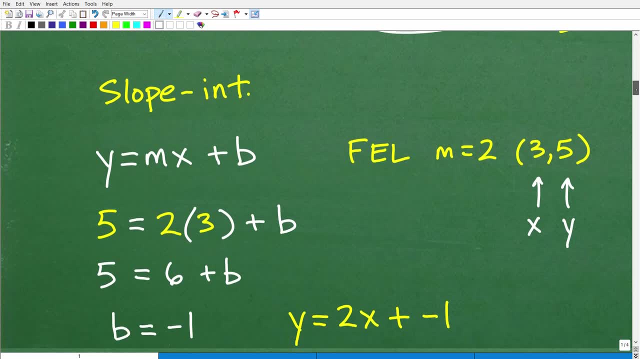 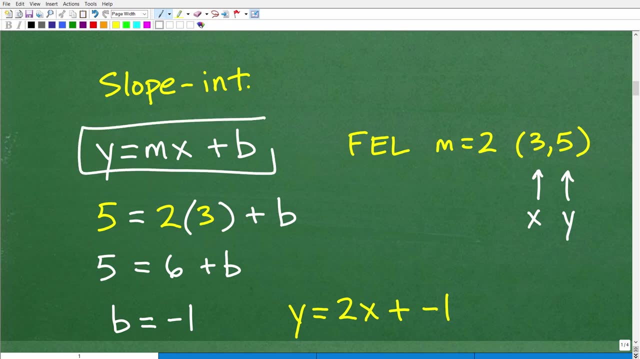 when you're not given the y intercept, i would strongly uh suggest you use the point slope formula. okay, so we're going to go ahead and take a look at doing this problem both ways. okay, we're going to use both forms. okay, so here, y equals mx plus b is the one that's the slope. 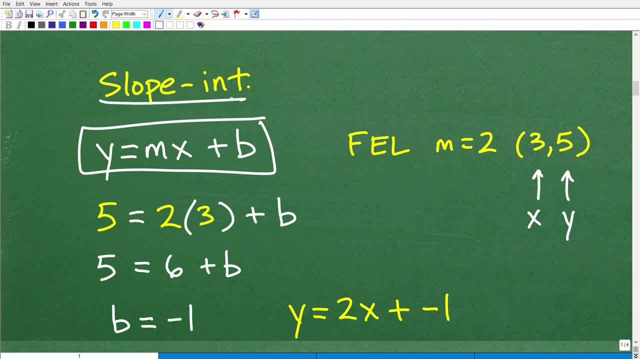 intercept uh, form of a line, okay, or formula. so let's go ahead and answer this question. so here it uh. the question is: find the equation line of a slope, of the line that has a slope of two. okay, so to use this formula right here, i need to have the slope m, i have that right here and i need 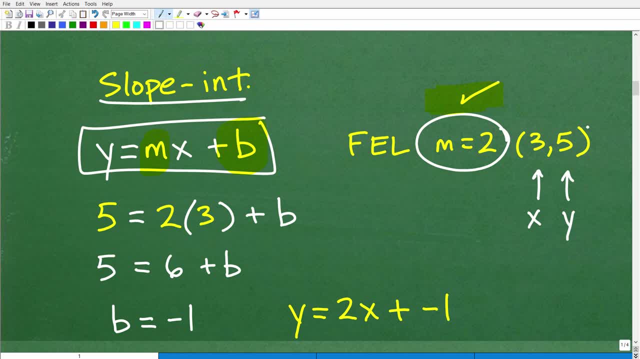 the b, the y intercept? i do not have that. what i have is one point. remember, to find the equation of a line, you need two pieces of information and you need this uh slope, and you need at least one point on that line. so i have a point there. 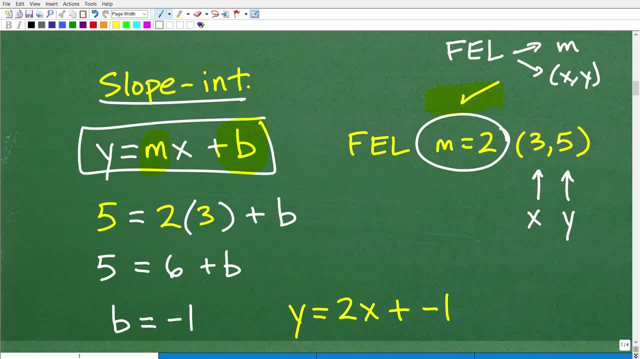 that's three, five. so this point, this x, this is an x- y order pair. okay, so this is x and this is y. so my x is going to be 3 and my y is going to be 5.. so, when it comes to this form, i have this, but i 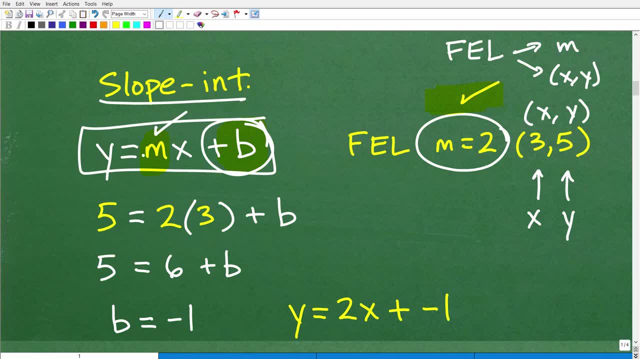 don't have this, and what you need to get a line in slope intercept form is the slope and the y intercept. so i have the slope, but i don't have my b or y intercept, so i need to solve for it. okay, so let's go ahead and show you how we do that right now. so we have y equals mx plus b, so y is what we're. 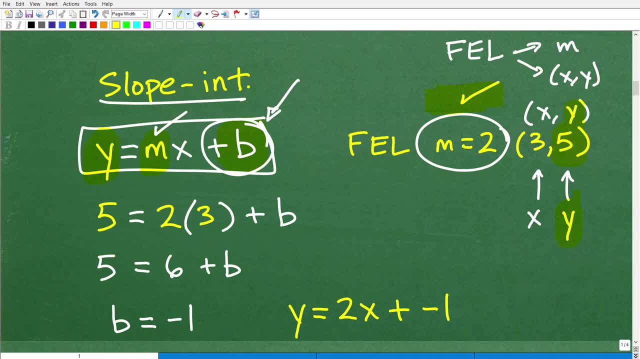 going to use this y right here, which is 5.. okay, we're going to plug that 5 in. m is 2, that's my slope. x is 1.. well, that would be my 3, okay, and then i don't have my b, so i have all my information. 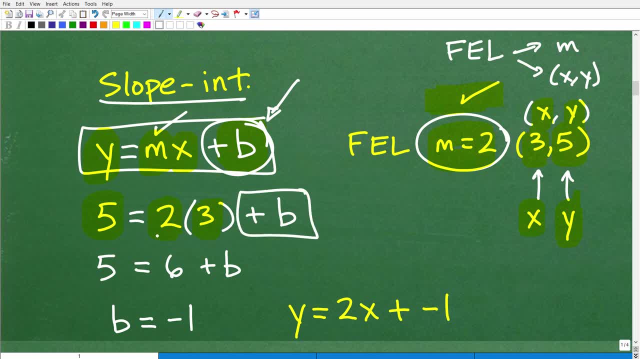 everything except for my b. so now i can solve for b. so 5 is going to be equal to 2 times 3, is 6 plus b. and then, when i solve for b, b is equal to negative 1, and simply subtract 6 from both sides of the equation. be careful what. 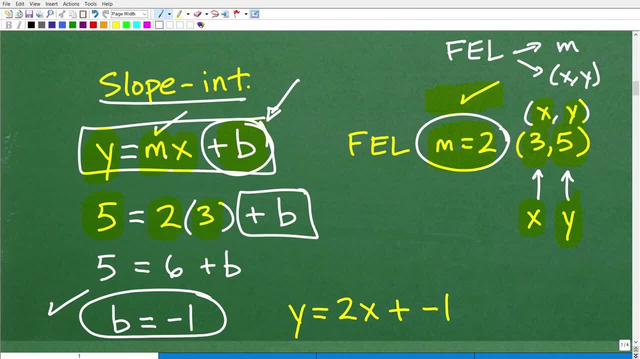 your positive negative numbers. so i have b is equal to negative 1. that's all i need. okay, i have my m. my m is equal to 2, so my y equals mx plus b. okay, m was already 2, so i'm going to plug that. 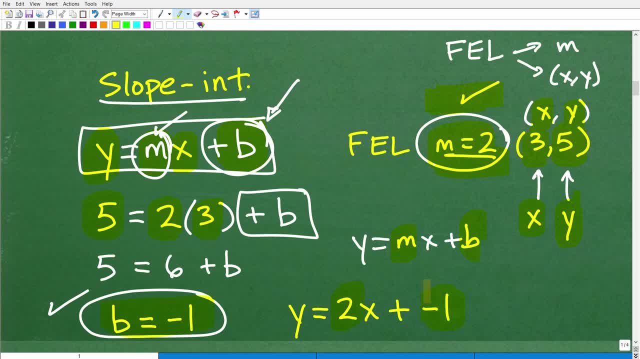 2, right there, and b i just solved for that's negative 1. and there you go. this is the answer. y equals 2x plus negative 1 and, by the way, if you're knew this already, you're like, yes, i could do this problem. well, let me go ahead and give you a nice. 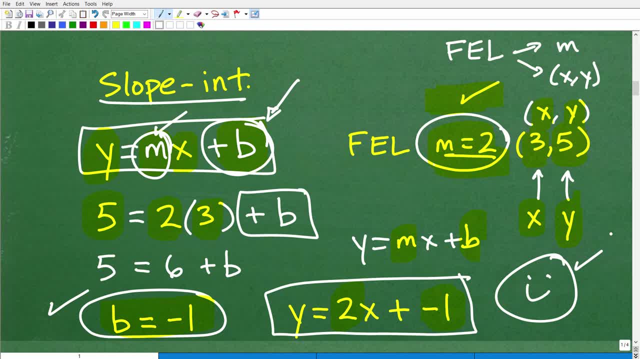 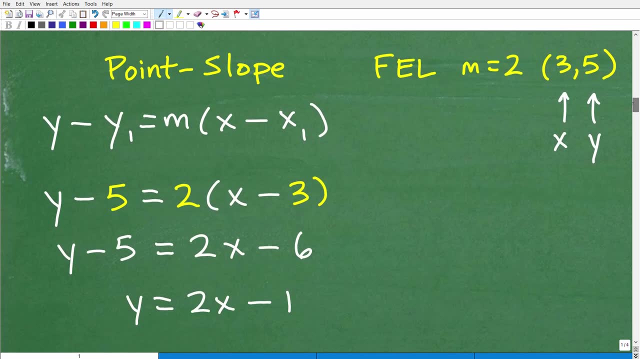 little happy face for being an excellent algebra student. so this is one approach, and this is not a bad approach. okay, but what i'm telling you is that you need to know how to answer the same question using the point slope formulas. that's what i'm going to show you right now. and for those problems, 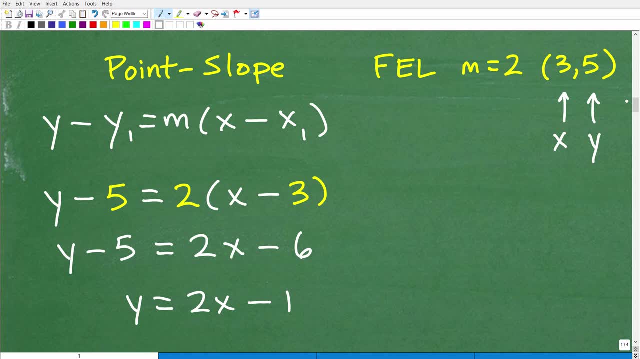 again that give you the slope and a point that's other than the y intercept. i would strongly suggest you use the point slope formula. so here is the point slope formula. let's go ahead and just quickly take a look at what we need to plug in. okay, so we have y minus y1. this is a value we need to plug in. 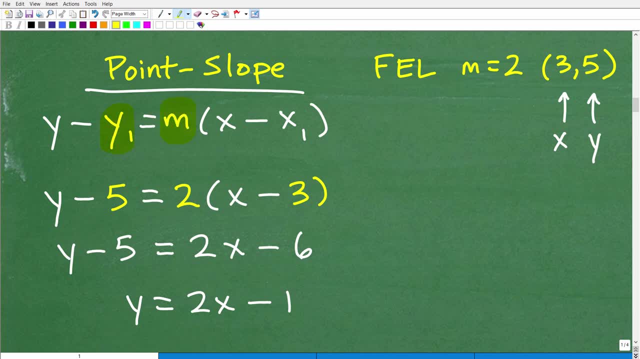 it's a y1, okay, or just a y coordinate. here is our slope. we need to plug that in and then we need to plug in right here for x. so this y1 and x1, remember, we're talking about a coordinate, we're going to do. 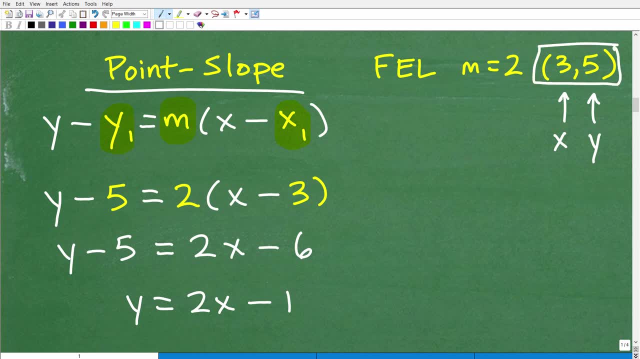 the same problem here. okay, we're just using the point slope formula, the. when you're given a point like: hey, the line passes through the point three, five. always remember these are a what we call an ordered pair. the first number is x, the second number is y. okay, it's a pair of numbers and 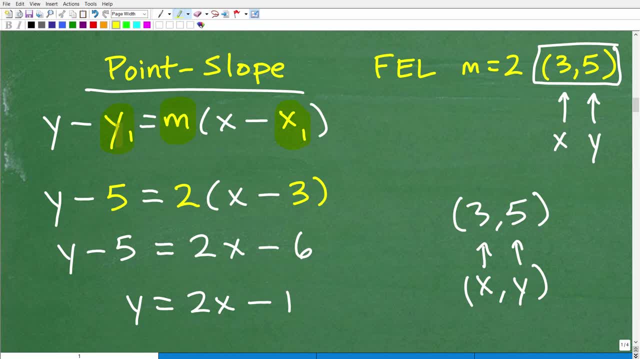 there's a specific order: x and then y, okay, so in this case, right here, y1 are, that's just our y, that's our five. this x1 is our three, right there, okay, then of course m we're given to as two, so now we just go ahead and just plug things in, uh, directly. 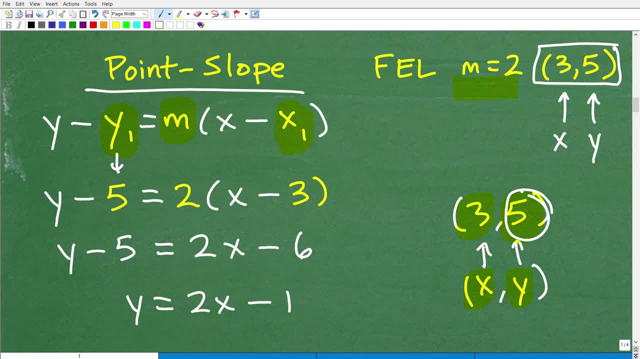 so y1- okay is our y value, which of course is five. so because i'm plugging it in m, i'm given the slope of m, that's two. so i put parentheses: x minus x1 is what my x value right here for my point. so that's three, okay. so at this time i just need to do this algebra. so first things, first two. 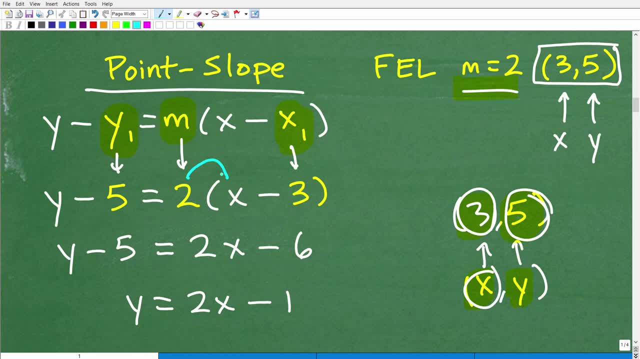 times x minus three. what you want to do is a distributive property, so that'd be two times x, that's two x, and then two times this. negative three is negative six. we have y minus five is equal to two x minus six. you want to solve for y. i'm going to add five to. 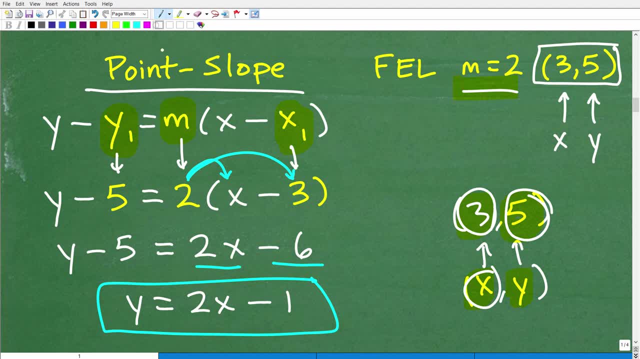 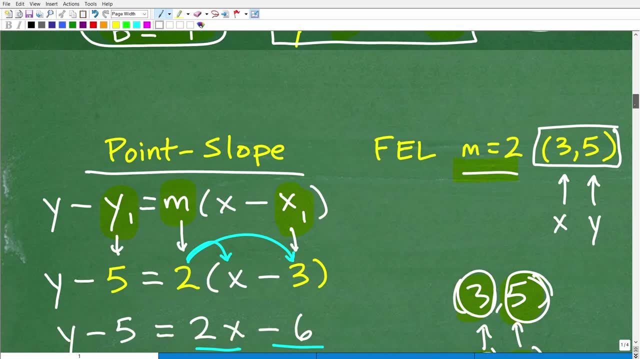 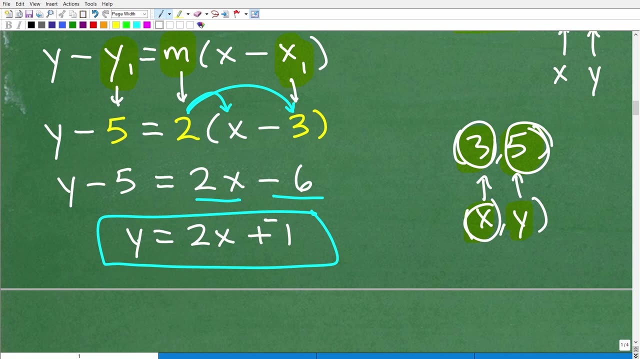 both sides of the equation. and here is what i get. okay, i get: y equals two x minus one. that is the same as y equals two x plus a negative one. because remember right here, uh, you might be saying those are different. no, no, you can just say y equals two x. you can turn this into a plus negative, okay, so 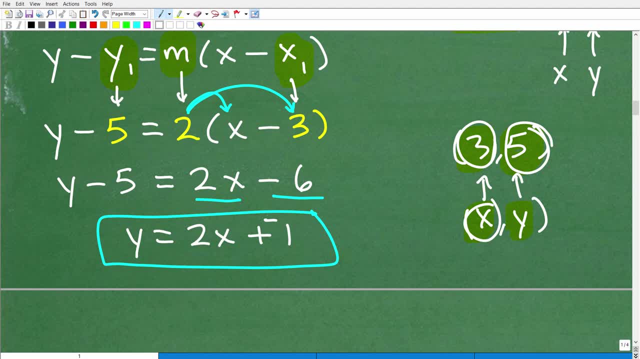 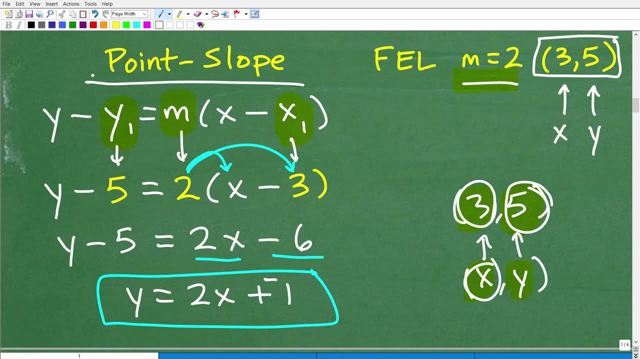 y equals two x minus one, or two x plus negative one. these are equivalent. okay, i'm telling you from experience. all right, most students when they get super good with that point slope formula, it's generally it's my recommendation that you use this as like your plan a. okay, when. 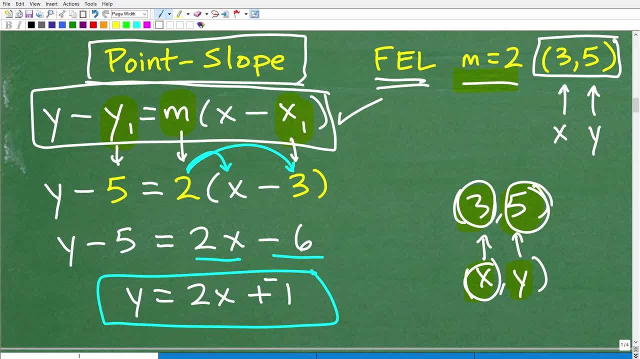 you're answering these type of questions, find the equation of the line. i will always kind of recommend that students go with the point slope formula. they just typically tend to do better with it in terms of getting your answer. but let's take a look at our final answer here. y equals two x plus. 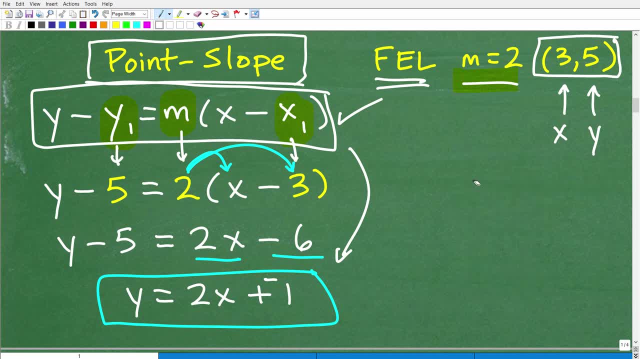 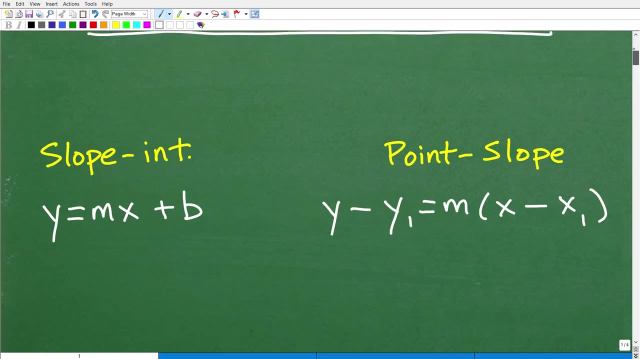 one. look at what's uh form? our answer is: even though we use the point slope form. our answer is: in y equals mx plus b form or slope intercept form. okay, so hopefully you know i did my job in this video and i gave you all the things you need to be thinking about when you're learning the. 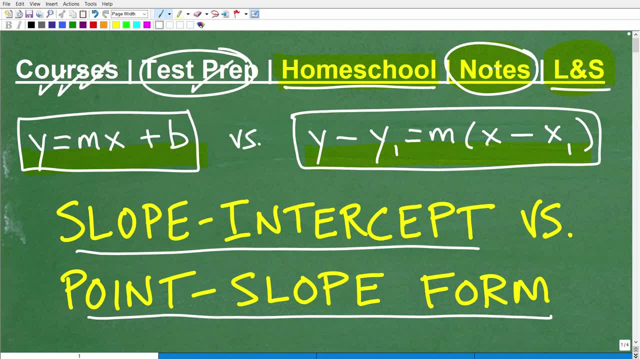 slope intercept and point slope formula. okay, it's a big topic because we're talking about linear equations, graphing lines, finding the equation of the lines, and there's different techniques you need to know, so just don't get stuck on one. you're like, oh, i'm super good with this and i'll.